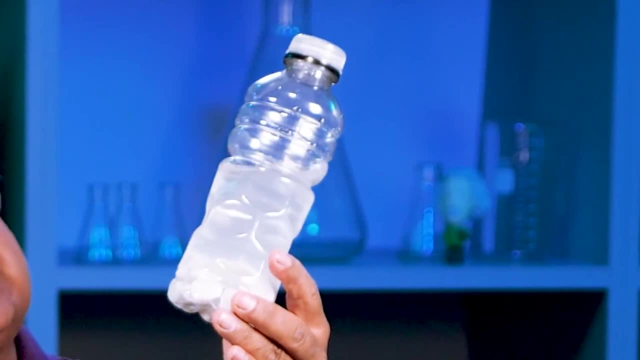 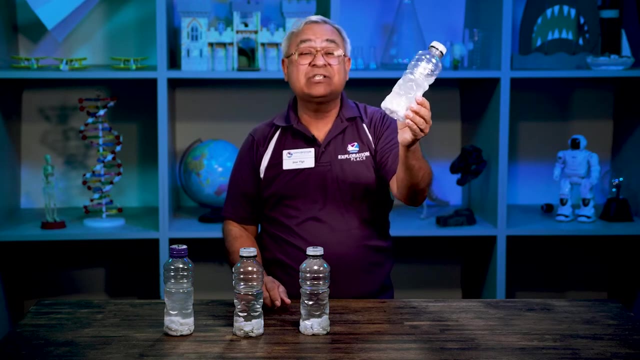 how come it's cloudy? What's causing that cloudiness? And hopefully you'll come to the conclusion that that cloudiness was caused because the rock is already starting to break down and turning into dust and it's clouding up the liquid. Now, if we do this 20 times- 1,, 2,, 3,, 4,, 5,, 6,, 7,- 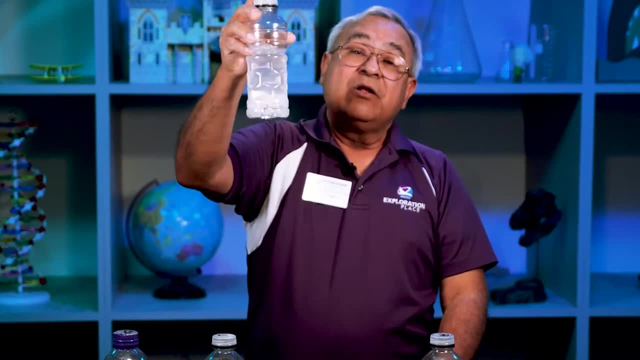 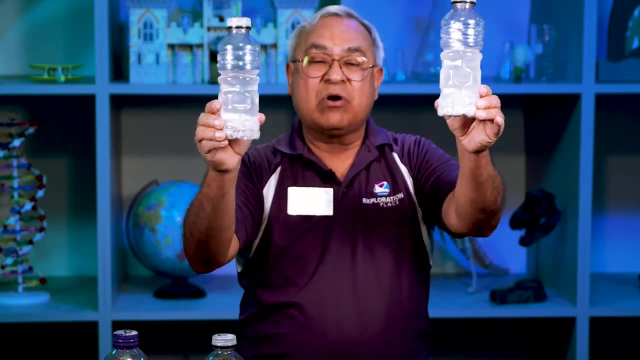 8,, 9,, 10,, 11,, 12,, 13,, 14,, 15,, 16,, 17,, 18,, 19,, 20,. we will also notice a little cloudiness, but when you compare these two bottles together, you'll notice one is more cloudy than the other. 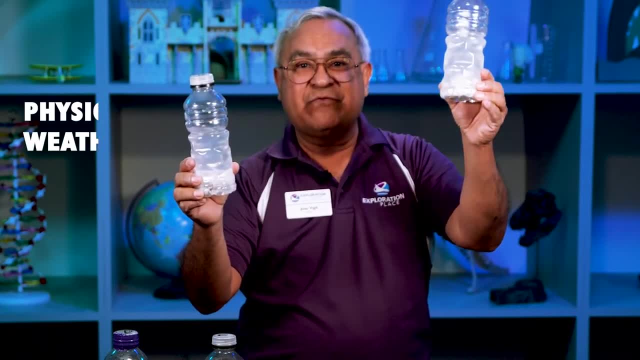 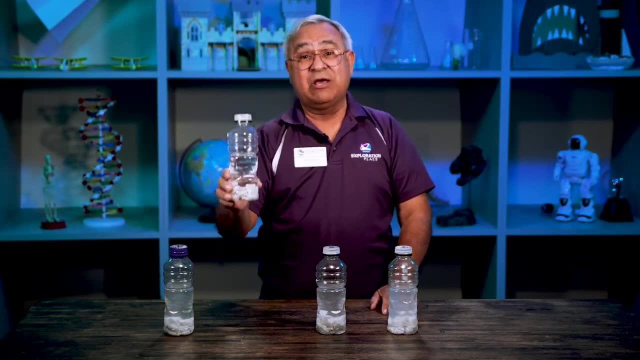 Now how do we explain that? That's because there's more physical weathering happening in this bottle versus the one with 20 shakes. Now we are not going to shake bottle C at all. In science we call this a control, because it's our comparison so that we can make. 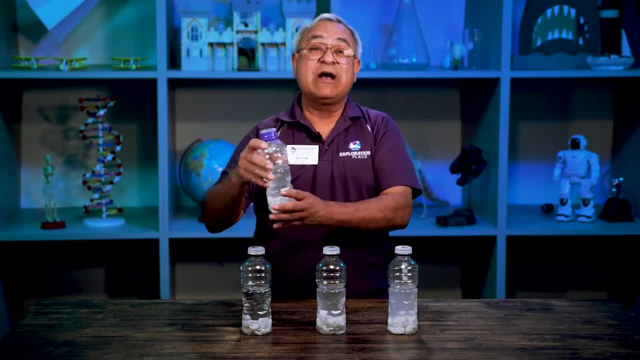 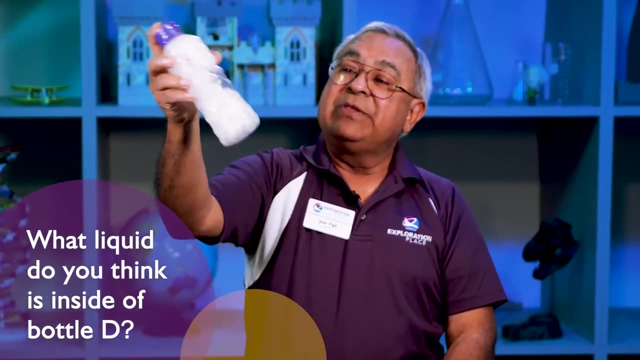 inferences and conclusions. Conclusions Now. lastly, I'll shake this last bottle, and I'll shake it only 20 times so that we can compare it to bottle B. Oh my goodness, Look at what's happening in this bottle There. 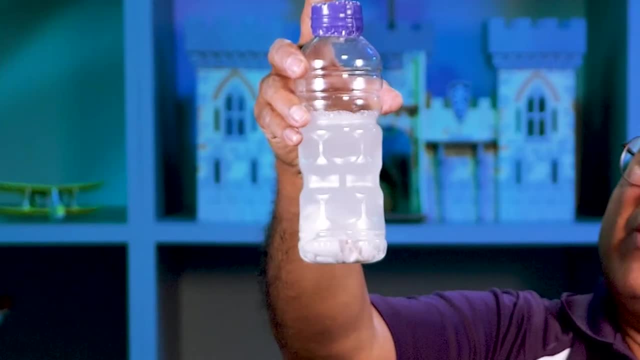 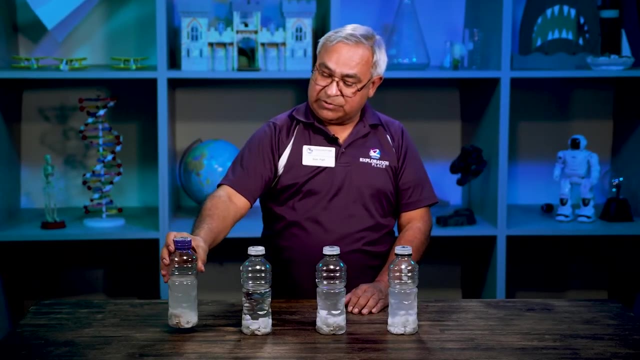 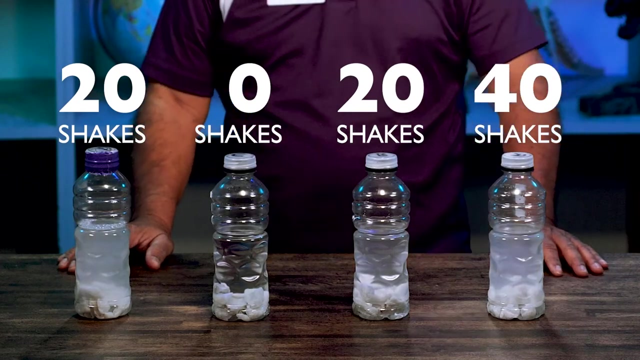 is a tremendous amount of action going on: bubbles, cloudiness, everything is happening at once in this bottle. And then, when we compare these bottles, we have to ask ourselves these questions: Which one of these is creating the most weathering the fastest? And hopefully you chose bottle D because bottle D not 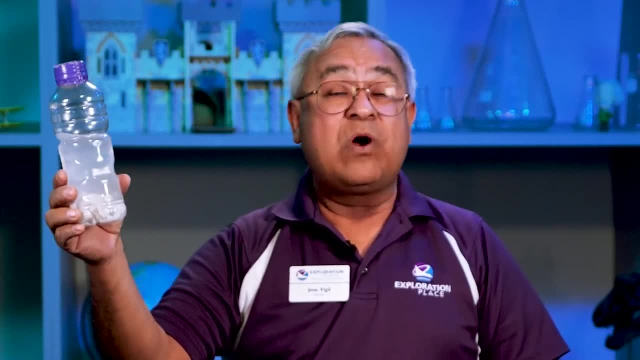 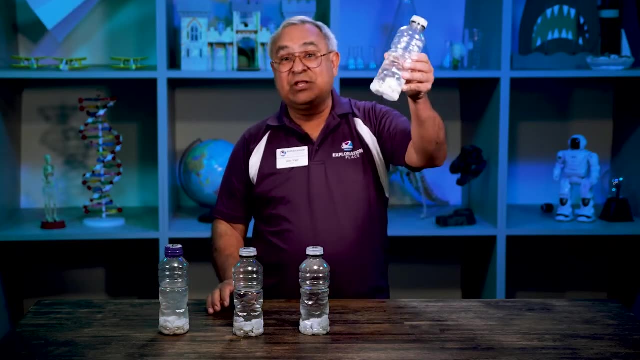 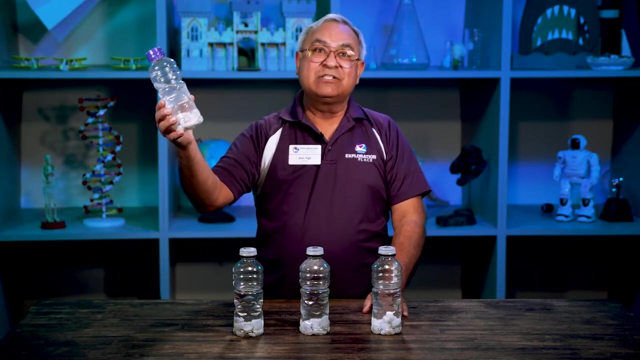 only had physical pounding, but it also had another type of weathering called chemical weathering. So what does that make you think? If you inferred that these bottles had water, you were correct. They have water in them. However, the last bottle has vinegar. Vinegar is an acid And I think a lot. 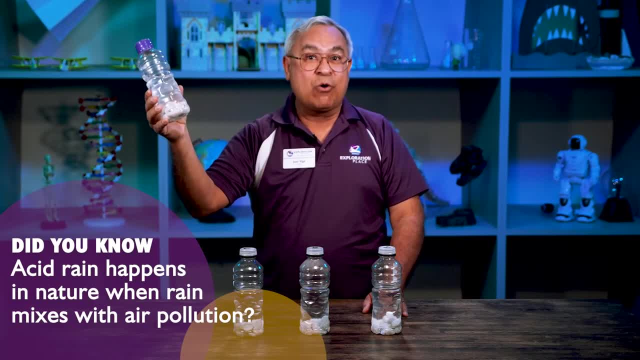 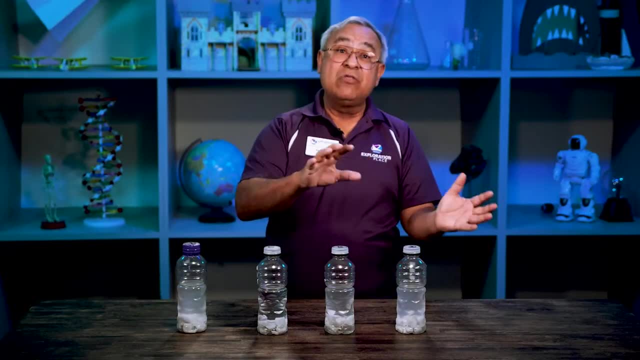 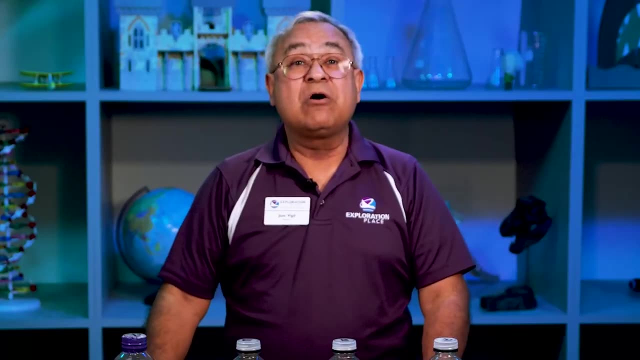 of you know that acids have a Yeah tendency to corrode or eat other objects. All the materials that are created by weathering usually stay right in place, But when those materials get moved by either water or other factors like wind or rain, we call that erosion. So you can do this at home: Be a scientist.